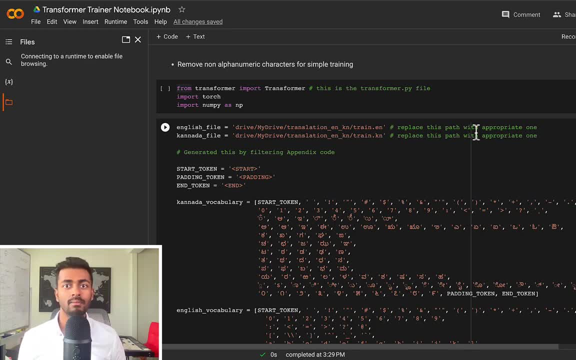 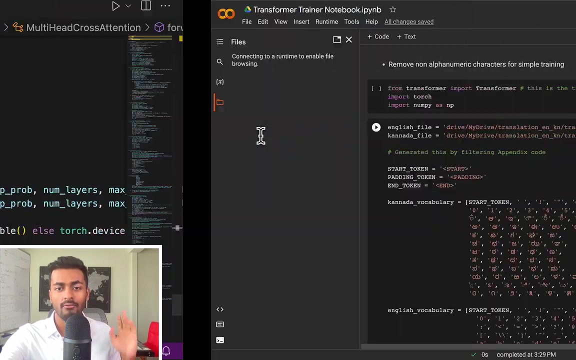 Hello everyone, and welcome to another episode of Code Emporium, as we continue our journey through the wonderful world of building a translator using a transformer neural network. Now, in the last dozen videos, we have built the transformer neural network from scratch, and here is the code to prove so. So in this video, though, I wanted to actually go through. 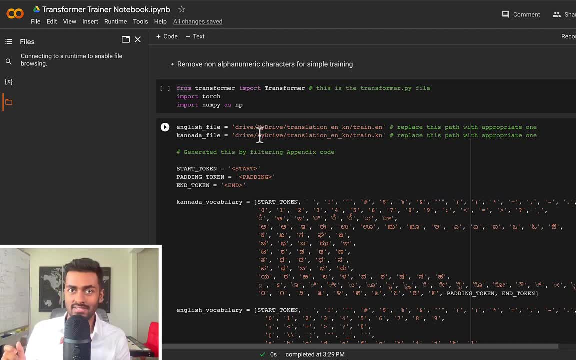 some of the inference translators that we get after actually training this model, and I also want to offer some insights of what you can do to build your own translator. If you want to see this entire code and with some of the data sets that I've used, I've uploaded. 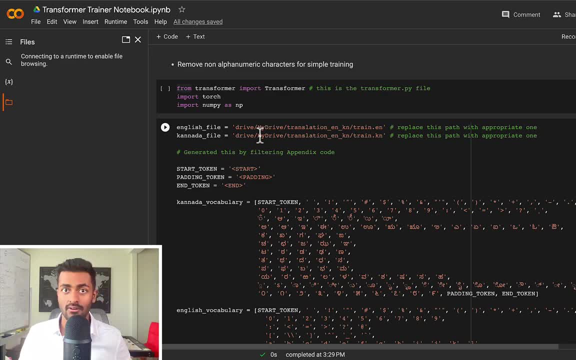 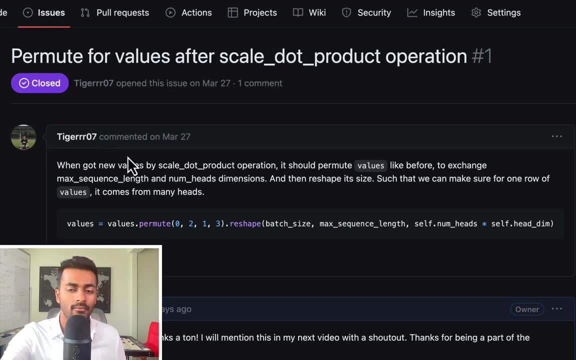 everything to github, and the link is in the description below. Before I get started with this video, I wanted to give a quick shout out to this user account, tiger07, where they helped point out a specific code that they used to build the transformer neural network. 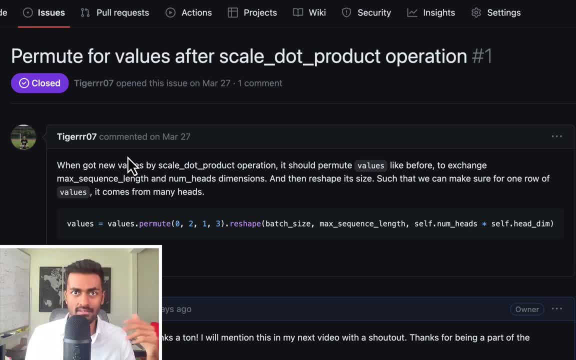 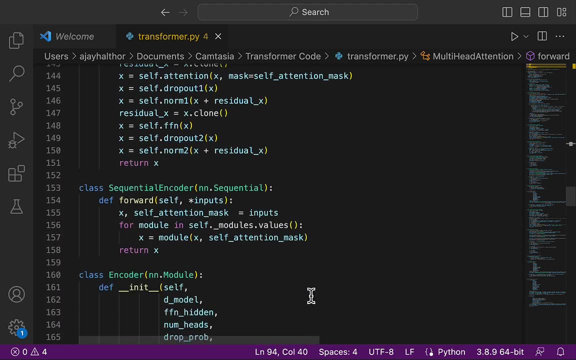 issue where in my last training videos for building out the transformer I kind of made some errors. they pointed out like two lines of code that I kind of needed to change throughout the network. and this is the line itself. it was just reshaping of these tensors, because I think it was pytorch when I tried to do I was just doing a values like some reshape. 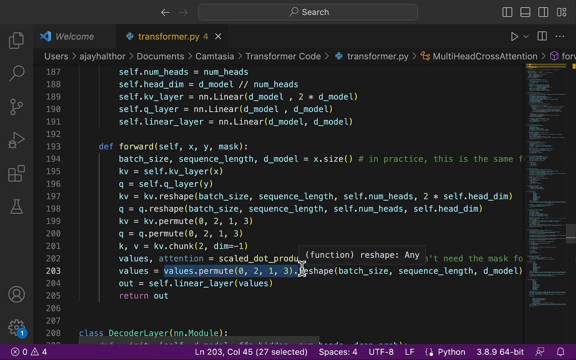 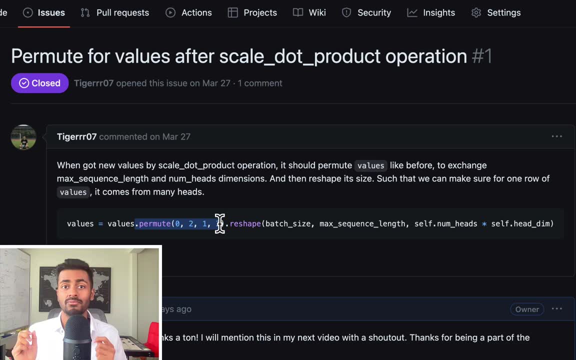 which would have completely discombobulated all my tensors. I needed to do a permutation of some layers and I was able to do a permutation of some layers and I was able to do a permutation of some layers. It's a very minor technical issue, but it was a major one in the sense that it stalled me. 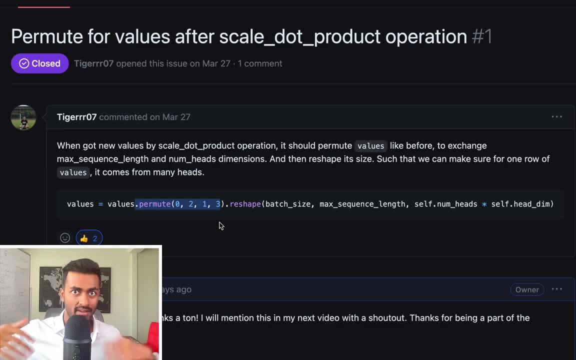 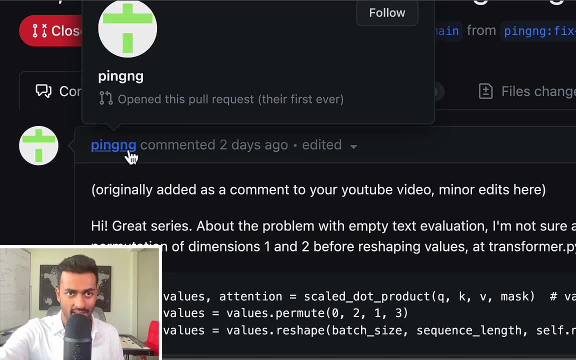 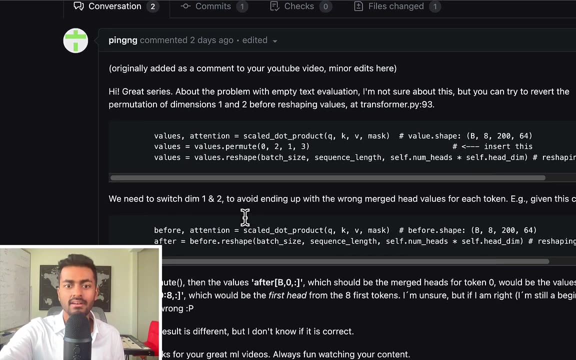 for a very long time and I'm really grateful that you know. when I reached out to the community, you all responded very well. I also wanted to give a shout out to this account, pingng. sorry for mispronouncing that, if anything. who recommended the same exact solution but also detailed why? 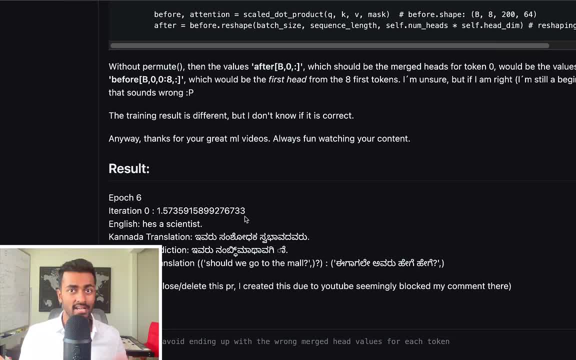 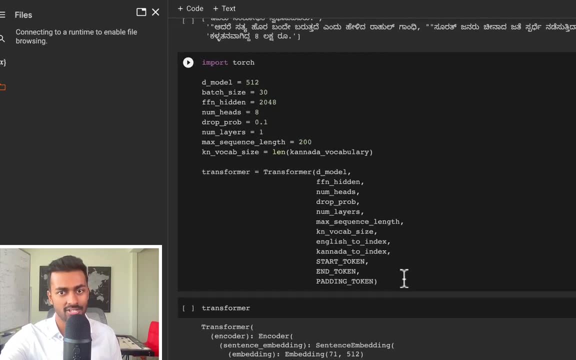 that was the case, so thank you so much as well, and that just shows how well this community does respond, because even slack nor chat GPT could really help me out, but you all did so. thank you so much. For now let's just go to the part where we're actually instantiating the 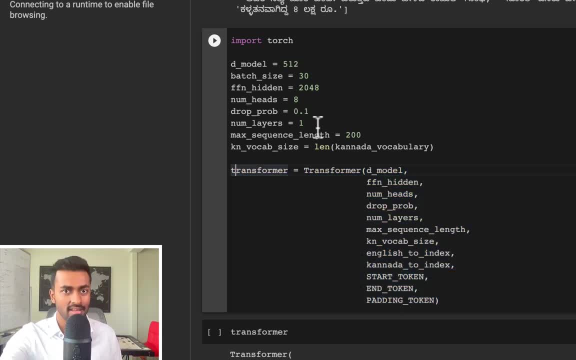 transformer, and the only thing I really want to point out here is that we are going to use only one encoder and one decoder layer, so this is going to be the simplest of the simplest transformer neural networks, so that it could just train this faster to see some reasonable results. 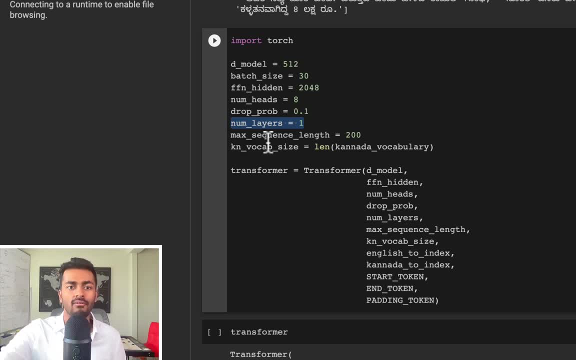 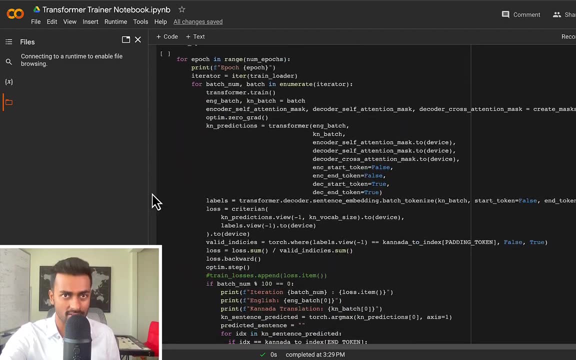 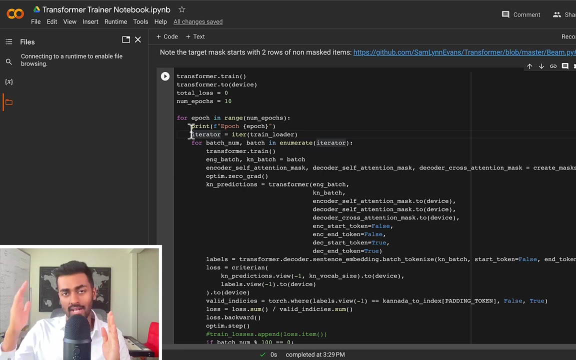 That's the only reason I did this and I did this training for about one and a half hours where I trained it for 10 epochs, where I'll scroll here. you see, that's 10 epochs, with the data set of around 200,000 English sentences to translate into a language called Kannada, and all of this. 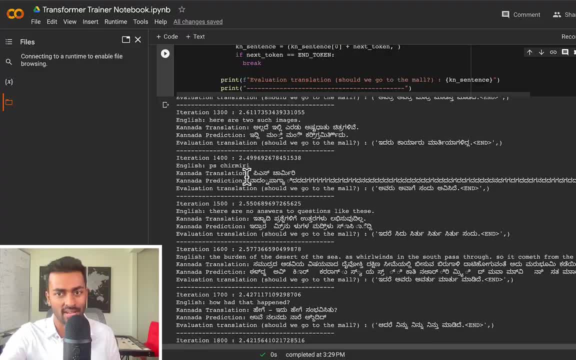 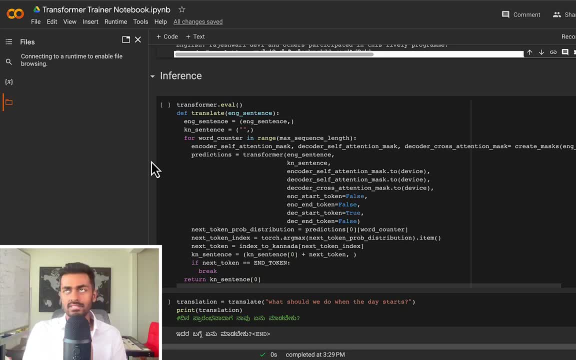 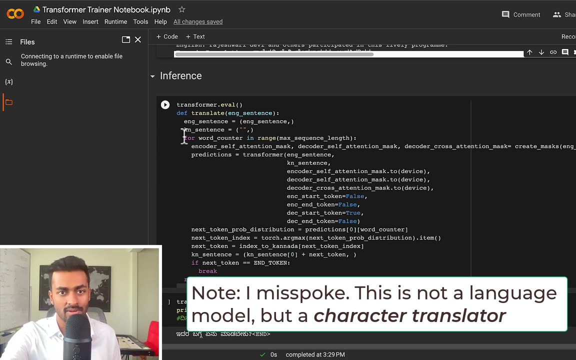 training epoch. I've printed out 100 epochs at a time. For now let's get to the good part of transformer. Let's get to the inference. So this here is a character language model where we're generating one character at a time, and so you'll see, everything is going to be within a for loop, where I am. 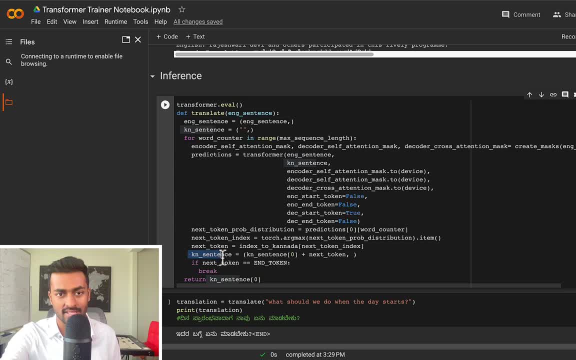 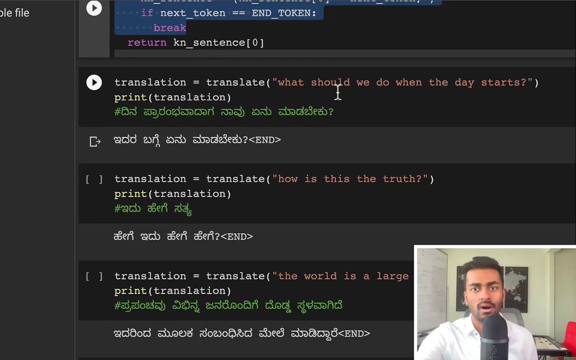 generating one character at a time. you generate the token and append it to the sentence and just keep doing this until you generate an end token which will signify the end of a sentence. On doing so, you'll get a few examples, so let's just look at a few of them. when I say- to try to translate what, 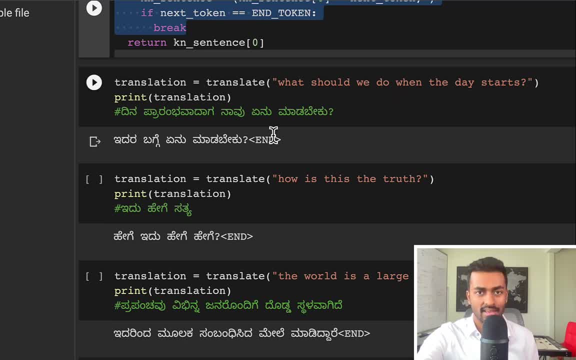 should we do when the day starts? The translation it gives is this sentence over here, which says: idara bagge ye no marabeku, which is: what do we do about this? although it doesn't translate exactly to you know the sentence, at least we can kind of see that there are some commonalities that are 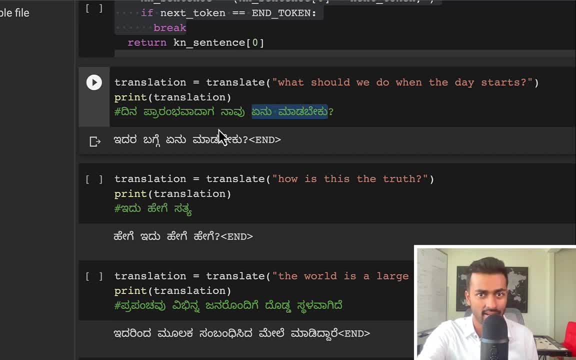 retained, like this last two words over here and these last two words over here. it is retained in some way. So ye, no, marabeku, That's these two words. that just means what should we do? and that just corresponds to this part of the sentence. So it kind of gets a part of the sentence right, but very clearly it distorts the. 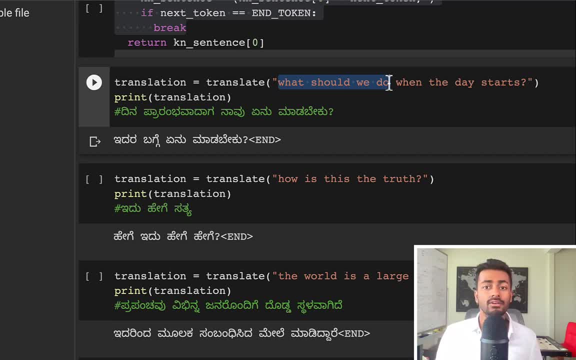 entire meaning, so it's not quite getting everything correctly. You can attribute this to a few cases. so the first thing is like the model is just too simple. it only has like one encoder and one decoder, and if you increase the number of encoder and decoder components you probably might be able to. 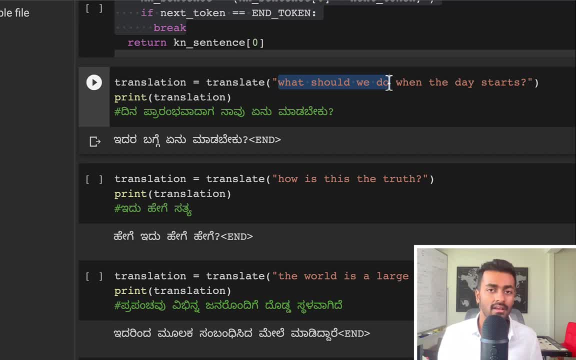 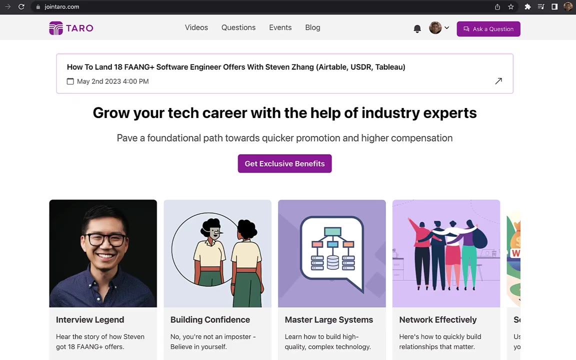 pick up on more idiosyncrasies in language. that's probably the biggest reason, but you can also try increasing your training set or increasing the number of epochs for your training time. before continuing with the video, i want to tell you about our sponsor, taro. this is a social platform to help. 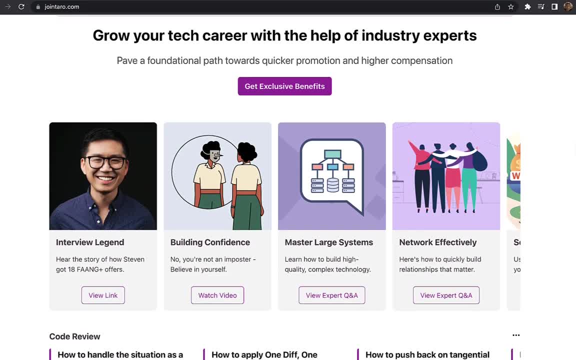 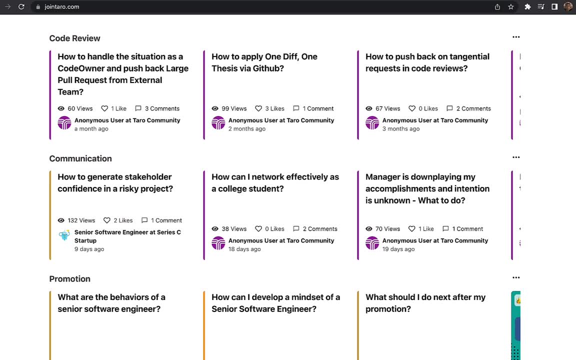 software engineers grow in their career. so, say, you land a software job. but then what? it could be really hard to navigate your career and it's tough to get good career advice. taro facilitates these discussions. whether you're a software engineer or a software engineer, or a software engineer or a. 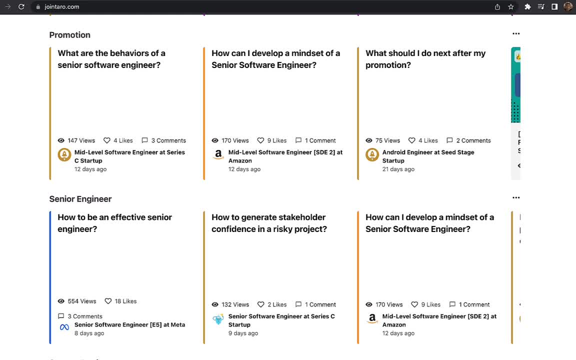 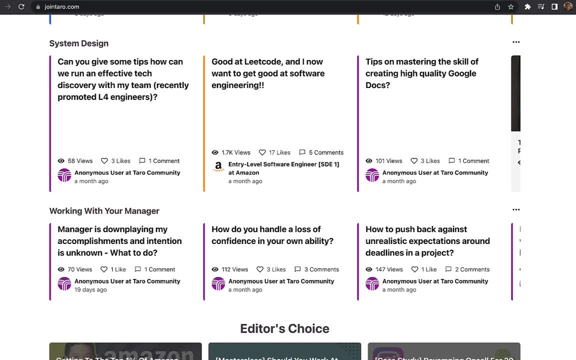 software engineer. you are an entry level or a senior. you can be a part of discussions to get advice from software engineers across many companies. there are many non-technical questions that i wish i could have asked someone in the past to advance my career, but really never found a good. 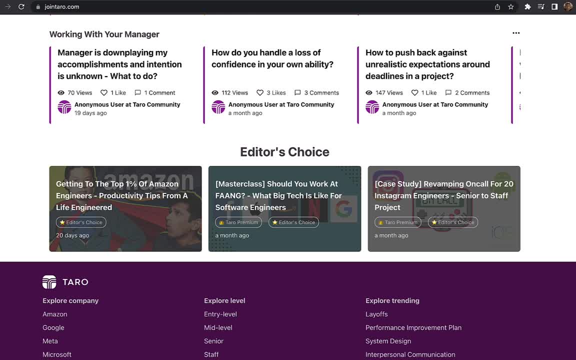 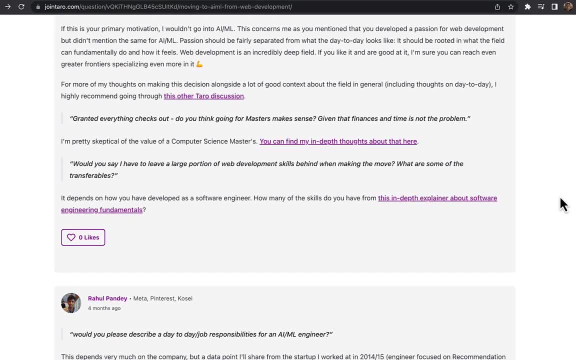 forum to do so, but i think taro is that good place. i'm a machine learning engineer, which does overlap with software engineers, and while the platform does not have too many machine learning engineering questions at the moment, i'm doing my best to help you get the most out of your career. 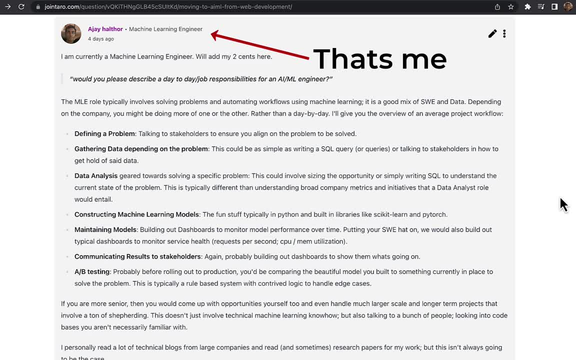 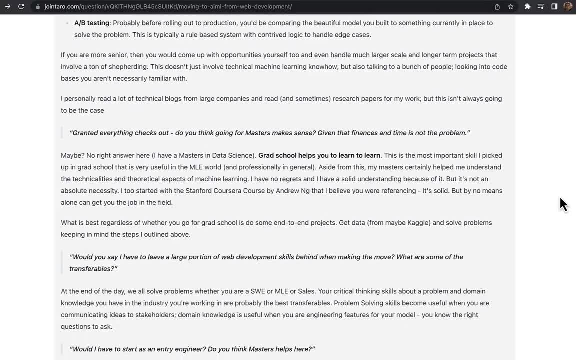 i'm really excited to answer any questions that are there still whenever i can, and i think this community is really nice to be a part of. still so, if you're looking for a premium community of software engineers to be a part of, consider signing up for taro using my link in the description to get. 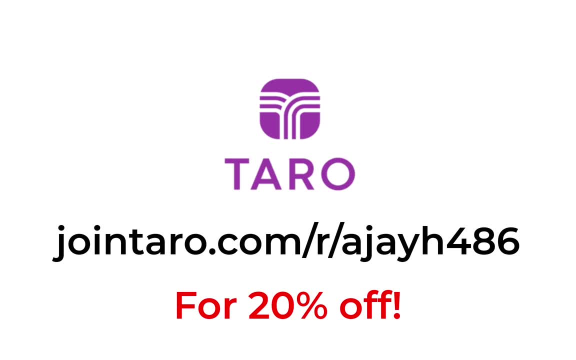 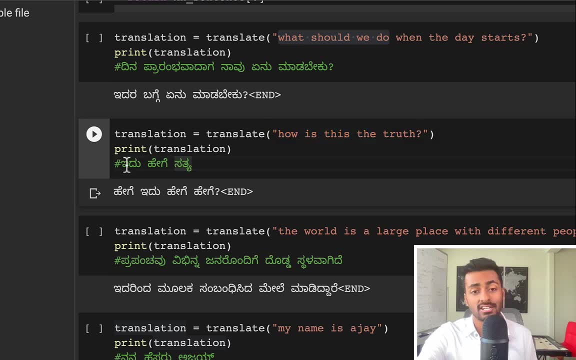 20% off your annual purchase. thanks for listening, and let's get back to the video now. the second sentence is: how is this the truth? the actual translation is, whereas this here is the generated translation, which is so this is not really a meaningful sentence, but you can see that there are some commonalities. 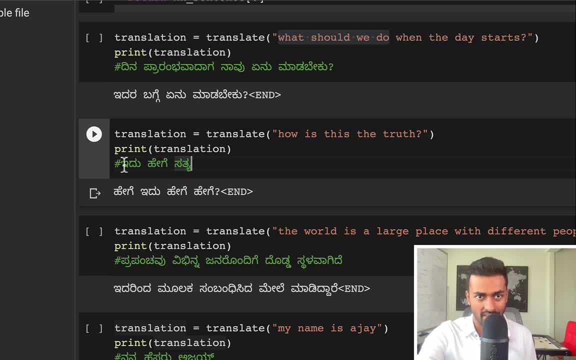 between them again. so you can see this um is generated as well. so it means like: this is how satya is truth. so in it translates to how is this the truth? so it does generate some part of it and you can see. just by looking at these two sentences you can see that there are a lot of 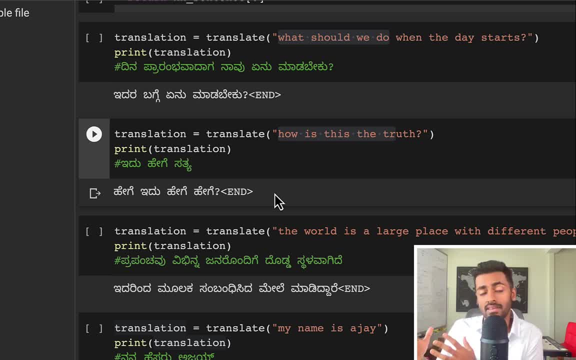 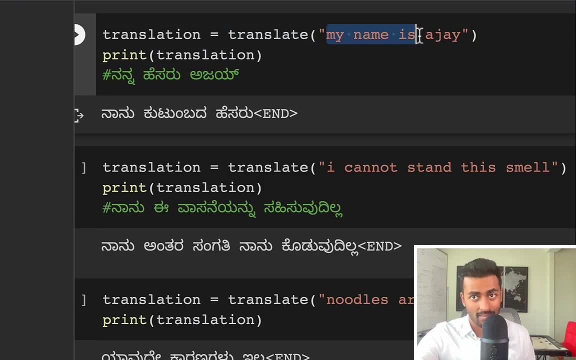 these two examples, you can kind of see that it is definitely learning something, although it might not be complex enough to pick up everything about these sentences now. this example is: my name is ajay, which should translate to nanna hesaru ajay, but it translates to nanu kutumbada hesaru, so you can see. 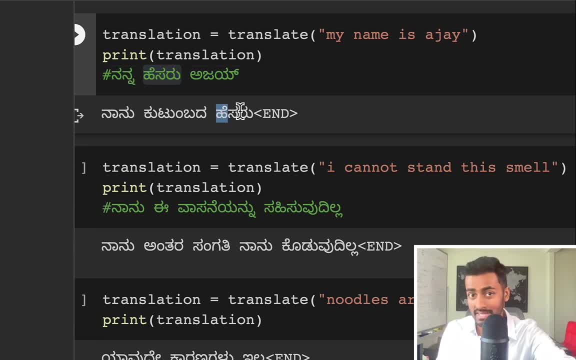 again, there are some commonalities with hesaru, which means name. nanna is my, but nanu is. it's very close to it, but it means me. it did not pick up at all on my name at all. ajay also, although the overall translation is off once. 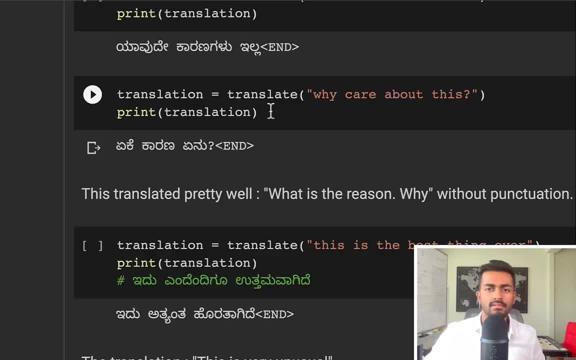 again we see some words that are actually common and correct. now this one's interesting: why do we care about this? the actual translation that it gave was with punctuation. it'll be like why? what's the reason? that would be the actual translation of this, which is actually very close to the to. 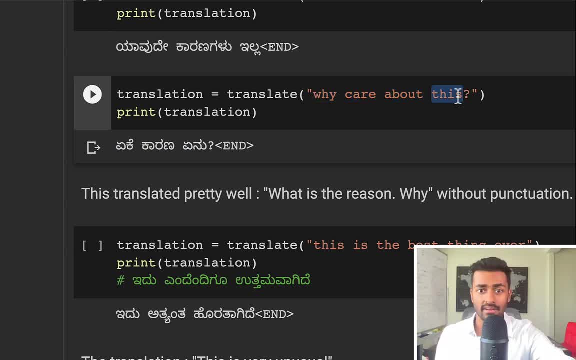 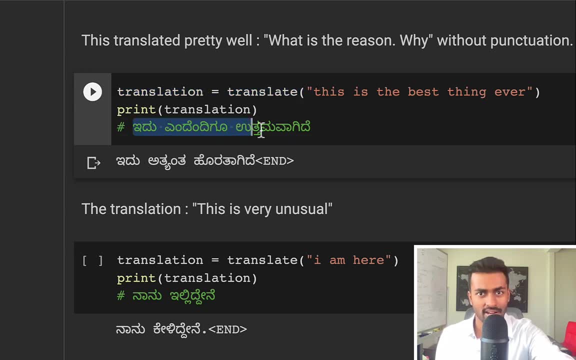 the translation of this initial sentence over here. so not bad, it did pretty good there. the next is: this is the best thing ever, whereas, you know, here it generates this sentence, but actual translation is this sentence which translates to. this is very unusual. so, though the the meanings are kind of off, you can see that. 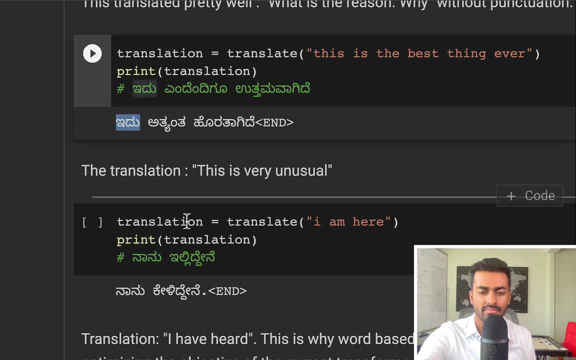 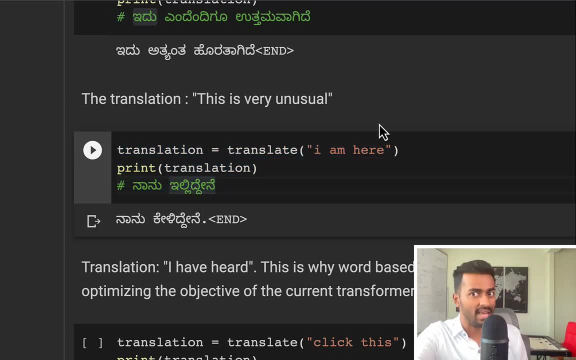 there are just some some commonalities between them. again now, this is probably the most interesting example throughout the lot where i wanted to translate. i am here. the actual translation is nanu illi dene, so projected translation by the translator was nanu ke li dene, so there are different meanings. this: 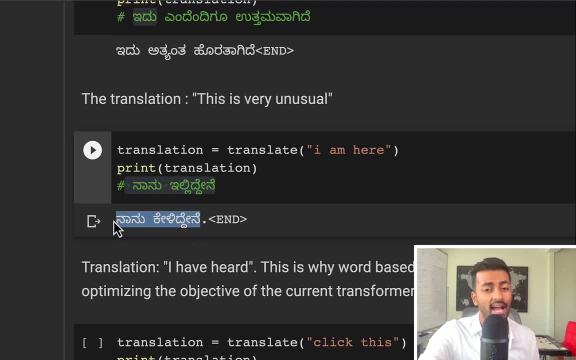 me, this means i am here, whereas this means i've heard something, and although there are different meanings, though, you can see that, from a character by character generation that this translator is performing, it's actually doing extremely well the only thing, in the translator's eyes, that it got. 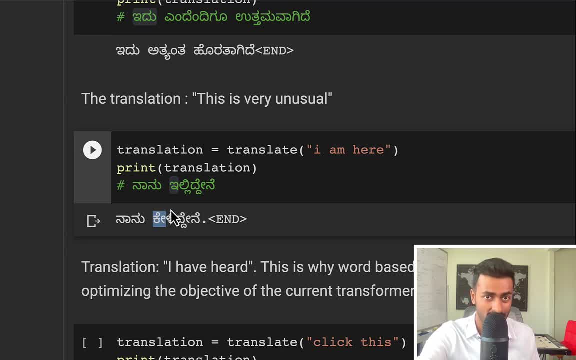 wrong was this eat and this k, like these two alphabets are the same thing, so it's not like it's like the only thing that are different in this entire translation, barring some small like la this, they're both laws, but either way, just one or two characters are the only things that are wrong. so 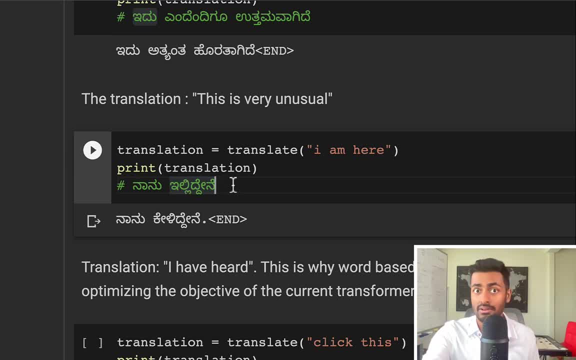 in the translator's eyes, this translation is actually a pretty good one, but this kind of made me think more about the fact that, okay, this is a character translation, but in general, word translations might actually perform better. but the the caveat of using word translations is that you're 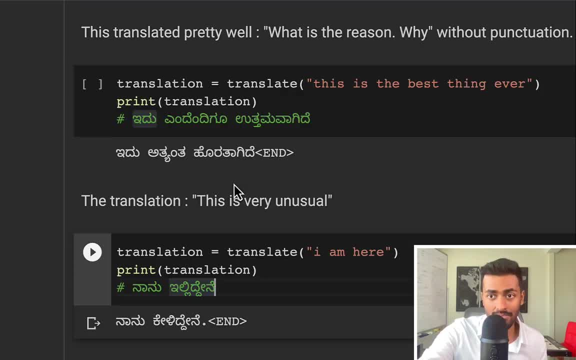 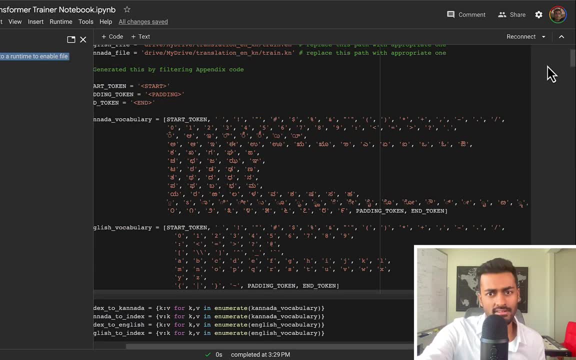 your Transformer will need to have a much larger vocabulary as opposed to what it has now. So you can see. if I scroll up to see like, what is the length of any possible characters that are possibly generated or tokens that are generated, You can see it's only a small set of values here. 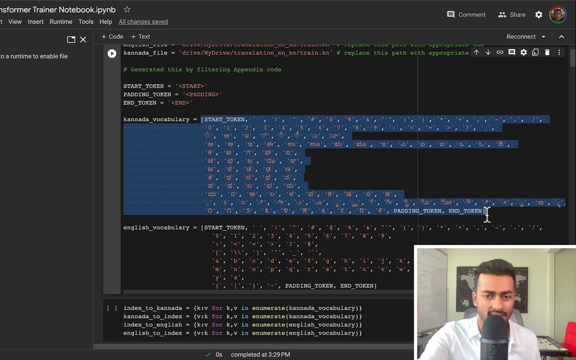 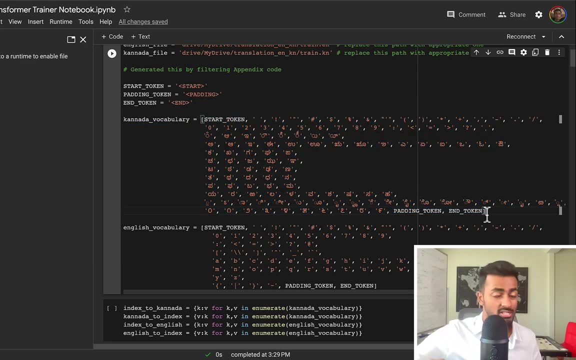 maybe, like you know, maybe 50 to 100 tokens or something like that, But if it was words, then all possible words were in this list. This entire list would explode to the tens of thousands, because there can be so many words that need to be generated. 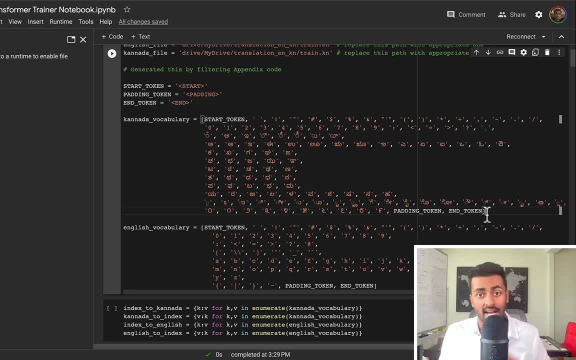 So there's always this trade-off between larger vocabulary size but interpretable values. So you need, like, much more complex systems, like you need probably a more complex translator and also way more parameters in order to account for, you know, words themselves. 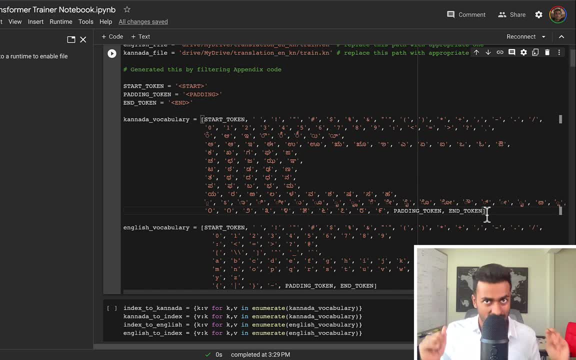 But with words, though, the sentence length will technically decrease. While here I have provided, like, the maximum sentence length to be 200 characters, the number of words in a sentence doesn't have to be like 200 words. It could be just, you know, a dozen or something like that. 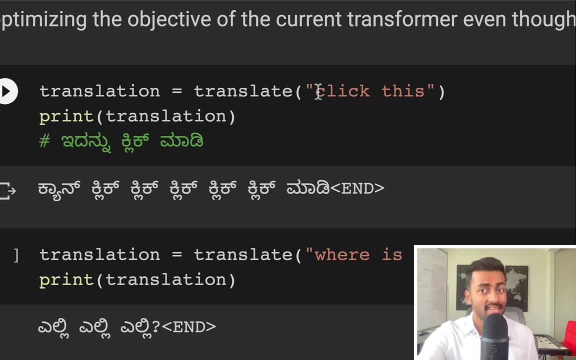 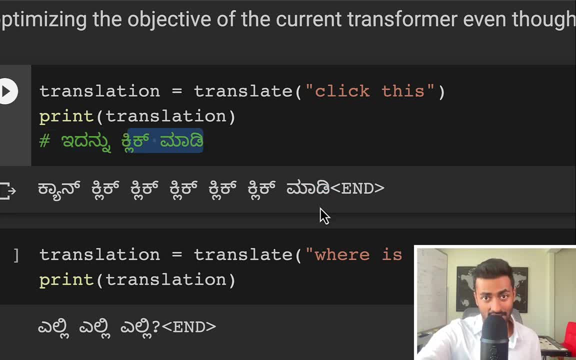 So, although it does get this last part right, Klik, mari, And it does get it here, It just loves klik, klik, klik, klik, klik klik. So it's just funny, But it is once again understanding what the task is, at least to an extent. 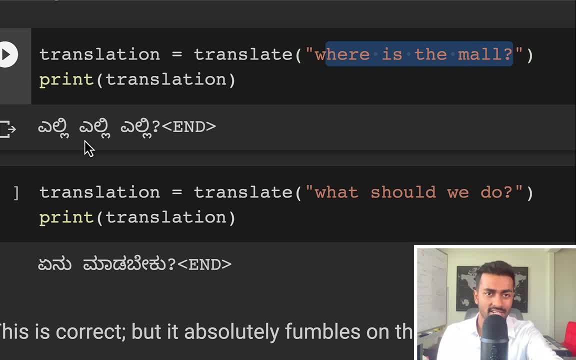 Now the same thing is here. Where is the mall? The translation is well, the translation that it generated was yeli yeli yeli, which is where, where, where. So at least it got the where part is, but it didn't generate anything else. 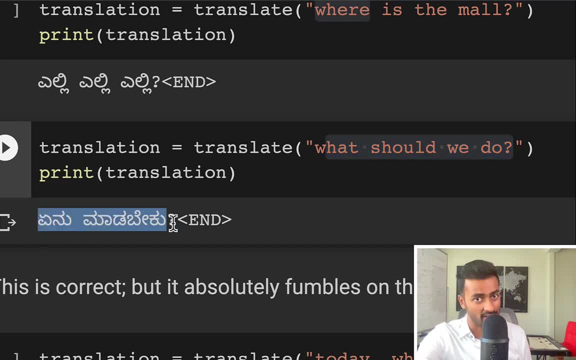 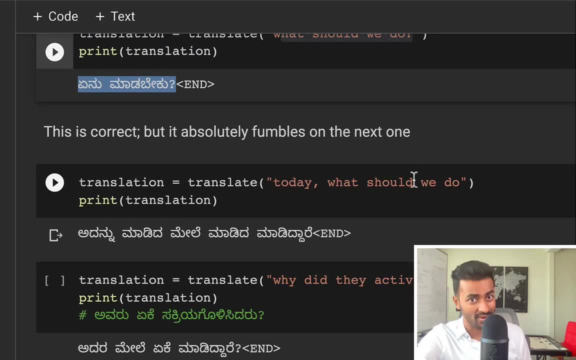 Now, what should we do? The translation is enu mari beku. Now it generated this correct, but it absolutely fumbles on this one here Today. what should we do This? I have no idea why it generates this. It says: 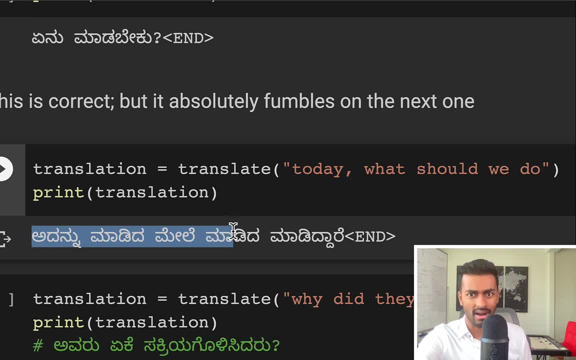 adhanu maridhara mele, maridha maridhare, So it just loves maridha mari is to do, And I guess that's like a very common phrase that you see everywhere, in both English and also in this language, Kannada. 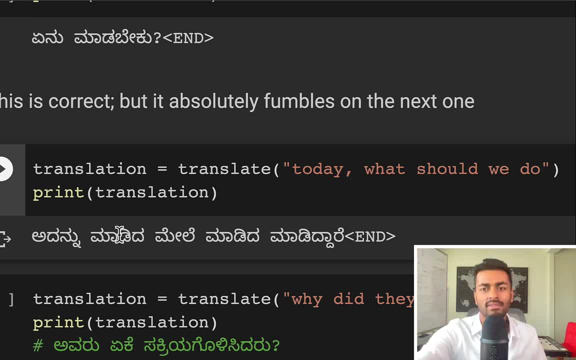 And that's why you're seeing like all kinds of forms. when you see like, oh, do, It probably tries to do mari, like every single everywhere, It just tries to to create this scenario, which, again, very interesting. 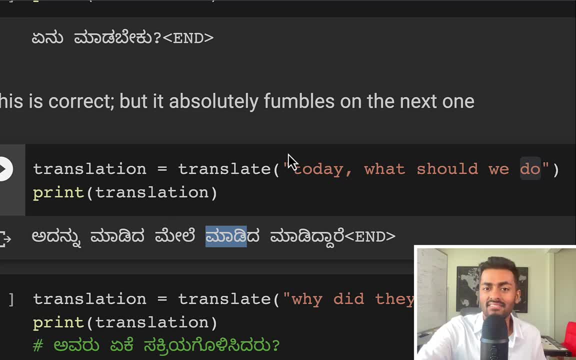 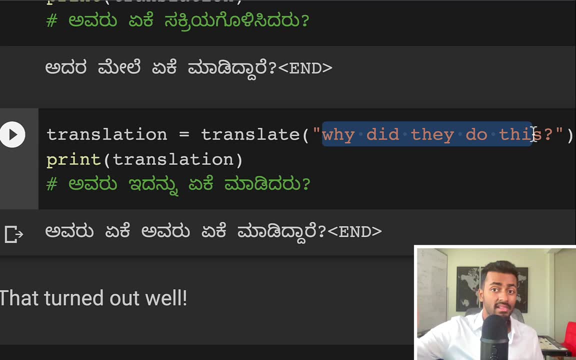 but it completely fumbles, despite. you know, in English, when we see this, it's kind of like the very same sentence as what we did before, just an extra word. So that's just a. it's an interesting note, But if I phrase it as, why did they do this? 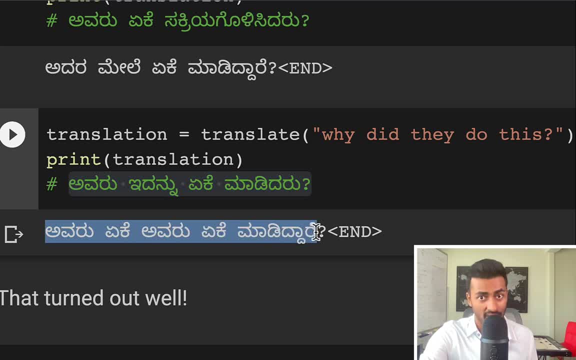 This sentence actually generated almost perfectly well, But again, this is something to do with doing something, So it's a very common common sentence in general, or a common phrase, So that's probably why it did so well. This last part here is also a very interesting one. 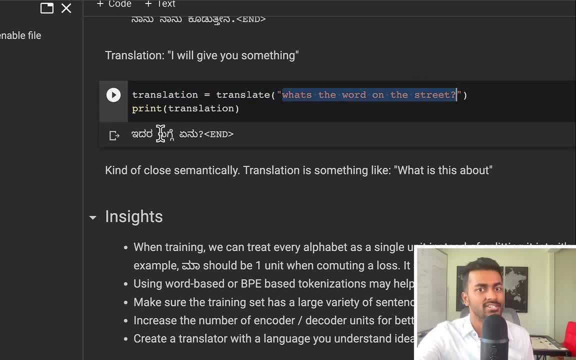 It's what's the word on the street And the generated translation is: so what is the topic of this, Or what is this about? is the translation which kind of does semantically relate to what this actually means, this little idiom here? 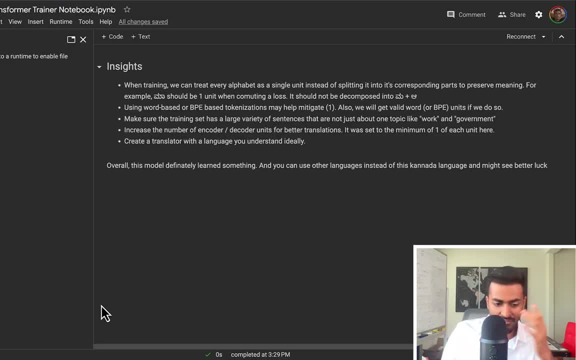 Let's now go through some insights where I'm probably going to give you some information And some tips when building out a transformer on your own with any language. So first of all, I want us to say: create a translator with a language that you understand ideally. 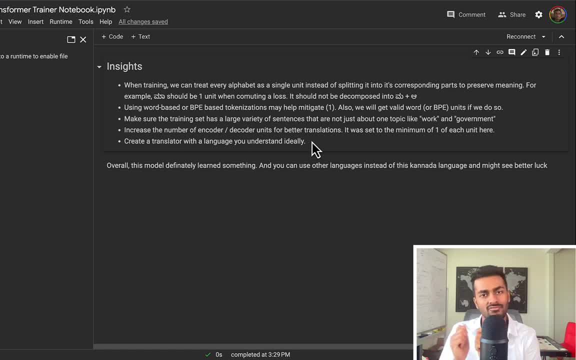 because it's just so much easier to see where the transformer is doing things correctly and where it's also doing things incorrectly. So generating that insight for yourself, I think, is very important, And you can better do so if you understand the language itself. 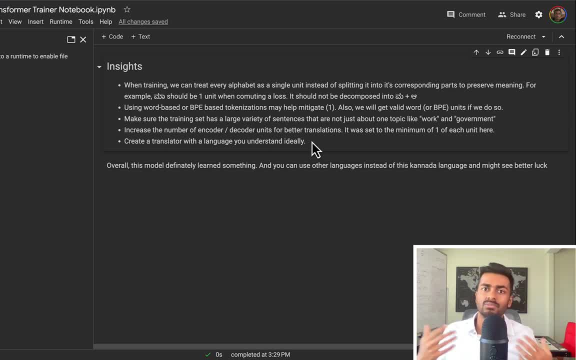 So in this case, people were saying: why did you use Kannada? It's because I can understand and I can properly evaluate it. Otherwise I wouldn't be able to come up with the insights that I did, Piggybacking off of that. 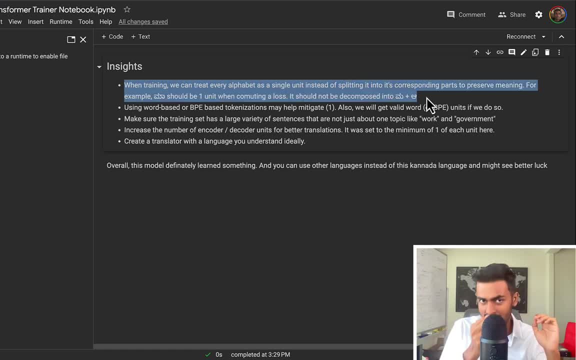 here's a, I think, a pretty important insight that I haven't really seen anywhere but I'll describe here. So when training typically, the English character set is known as what we call an alphabet, where every character kind of has a phonetic representation to it. 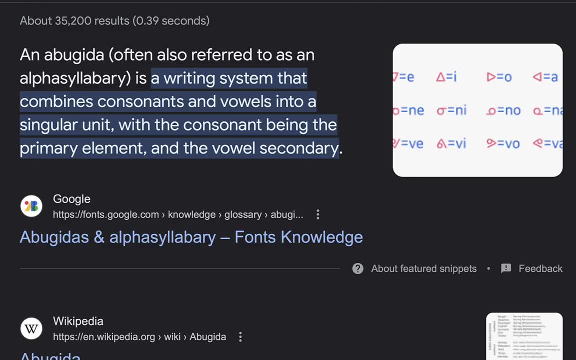 In a language like Kannada, it's more of an alphabet, a syllabary, So you have individual units to actually be complete like syllables themselves, And in doing so, that means that, even though, like, for example, this word, 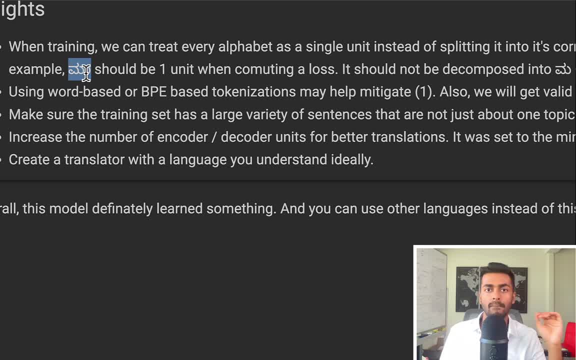 I think I typed it out here. So this is a character. This is ma Ma. if you write it out in English, it would be M-A, with, like you know, like an accent on top of it. That would be. 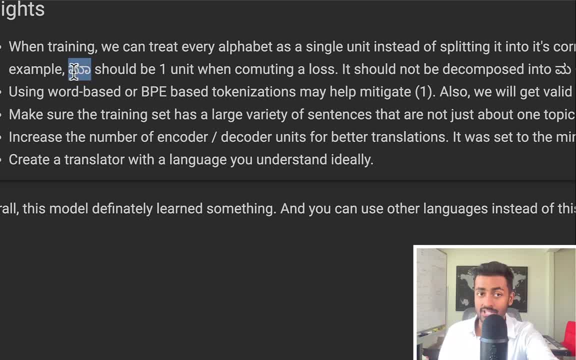 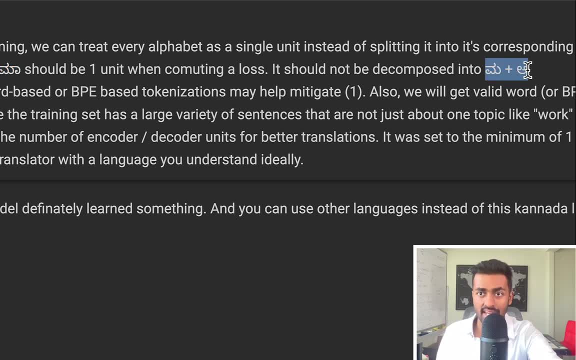 so it's like multiple characters in English, but it's a single character in the Kannada language. However, when I was dealing with tokens here, the way that I'm tokenizing the data is I'm also treating it as like multiple tokens. 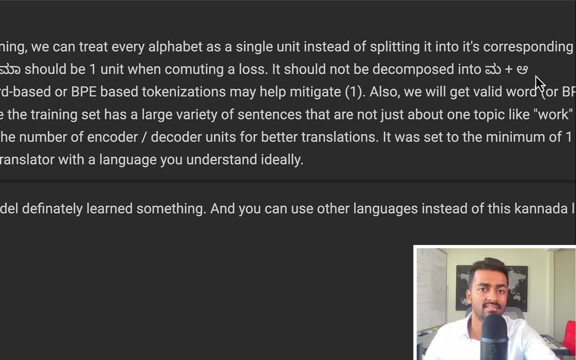 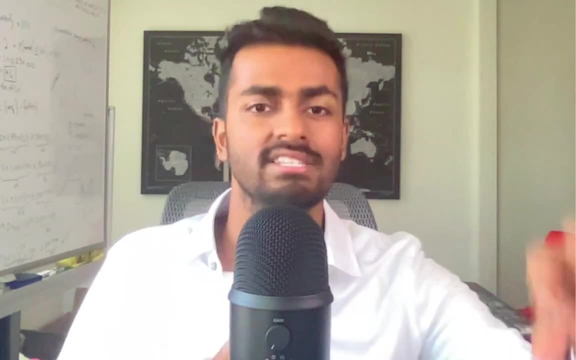 So it would be ma plus A. Even though in the current language it's actually supposed to be one character, I am treating it as two characters, And so what semantically just makes more sense is to create a tokenizer that will not just divvy up the entire. 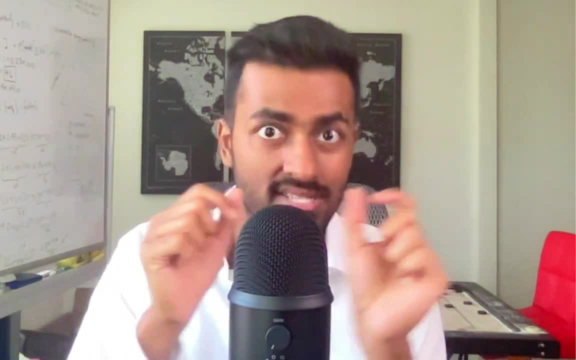 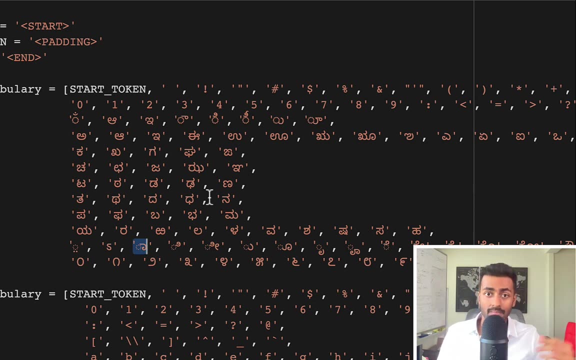 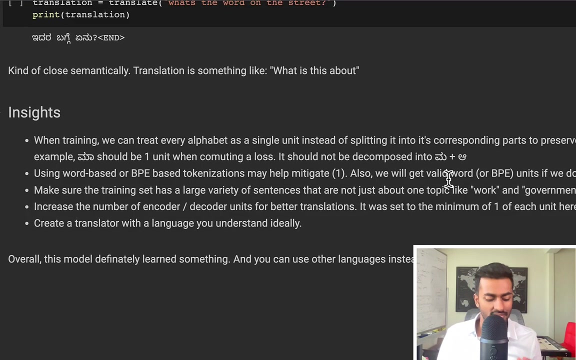 you know, Kannada like word into very sub characters, but rather divvy the Kannada word into actual Kannada characters themselves, which may or may not be a combination of two or more of these characters. Also, alpha syllabaries are a type of script. 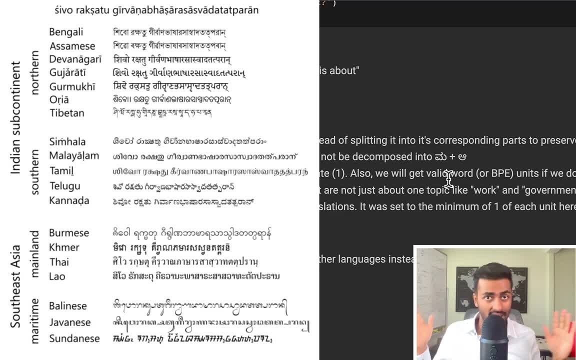 that are not confined to just this language, Kannada. There are many alpha syllabaries out there, And so just understanding the writing style may actually create a translator that is more meaningful, And so I highly recommend you try this out. Now, another insight that I mentioned. 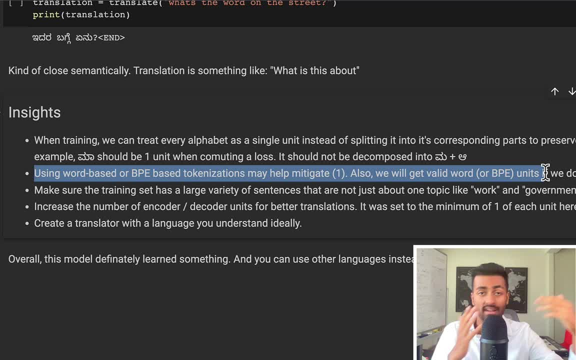 is kind of similar to what I described before. This is a generating one character at a time, So it's a smaller vocabulary but longer sentence length. but you can play with generating like word at a time where it'll have a much larger vocabulary. 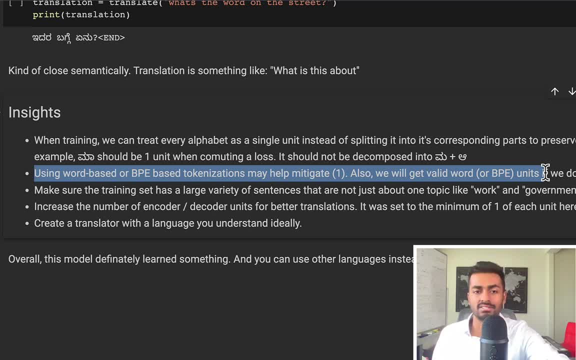 but smaller sentence length And a good mix of both worlds is to use something called byte pair tokenizations or byte pair encodings, which are like sub words. Now, the issue with this is that it's very hard to create a byte pair encoding for, say, 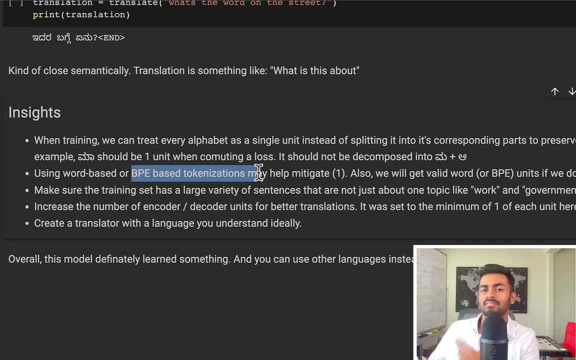 certain languages if they don't- you know, if they're not really don't have a great researcher online presence, So it's hard for me to find one for the language Kannada, And hence I went with character tokenizations for now to illustrate concepts and ideas. 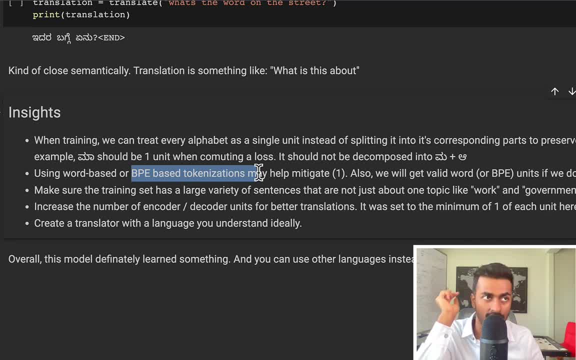 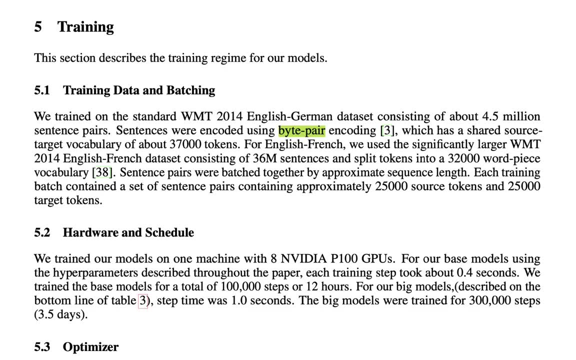 But if you're able to create like byte pair encodings for your languages input and outputs, then I think that might be like a good starting point. In fact, I think this is exactly what's happening in the main paper and a lot of other research associated with generative models these days. 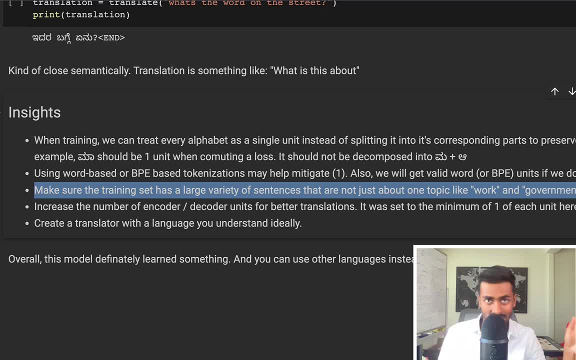 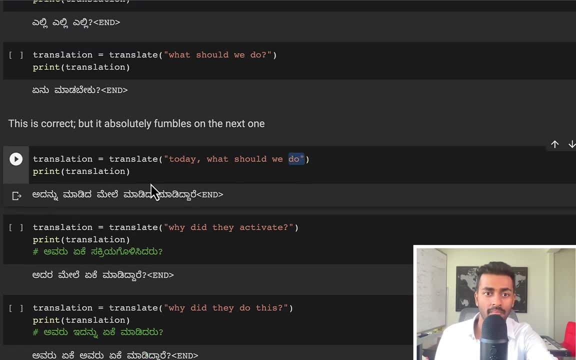 Another one is to make sure that your training set has a large variety of words in general. You could see that above when I illustrated here there's a lot of sentences that are like to do right, Marty is there's like a lot of these sentences. 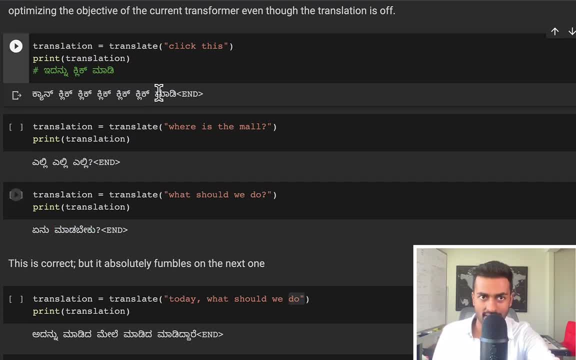 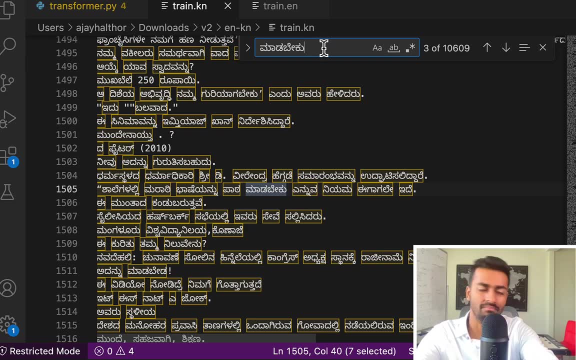 that kind of go and Marty over here. In fact, if you look at this data set, there's actually 10,000 cases at least, of like. there's like millions of records here, but there's like 10,000 cases at the very least. 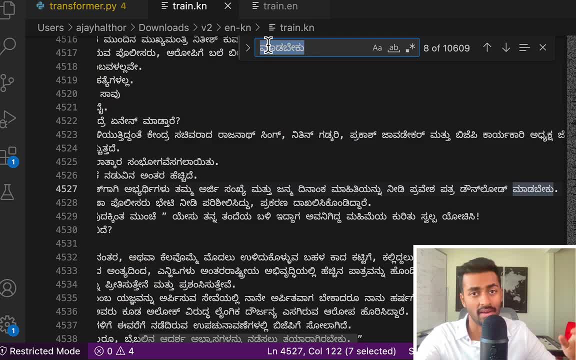 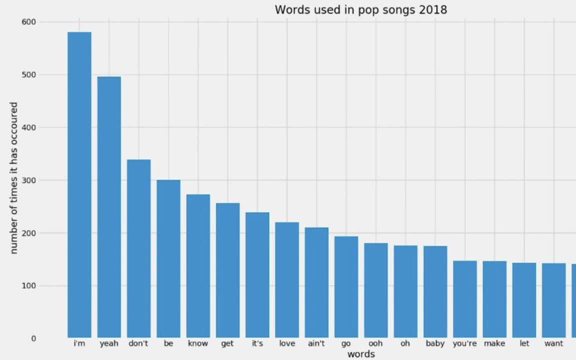 So I would suggest you try to plot out every single word and their frequency counts, just to get an idea of what kind of data set you're dealing with, whether it's very catered to like news, government articles, politics, or if it's catered to just like general and random sentences. 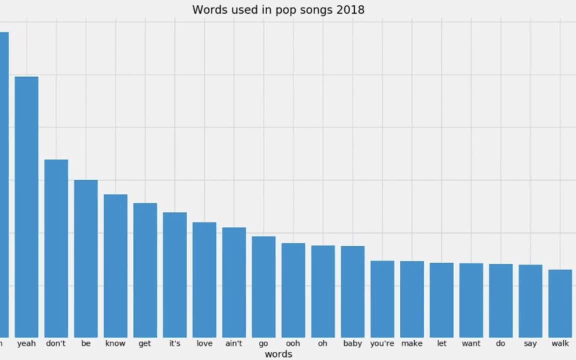 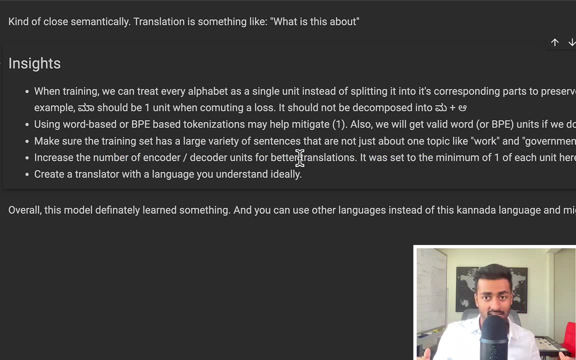 which ideally would be the case for general translators. And the other one is just more technical, where you're increasing the number of encoder and decoder units, As I've only used one, keeping it very simple, but you can ideally try with more encoder decoder units. 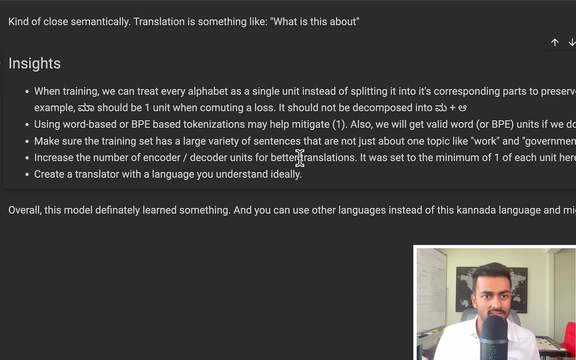 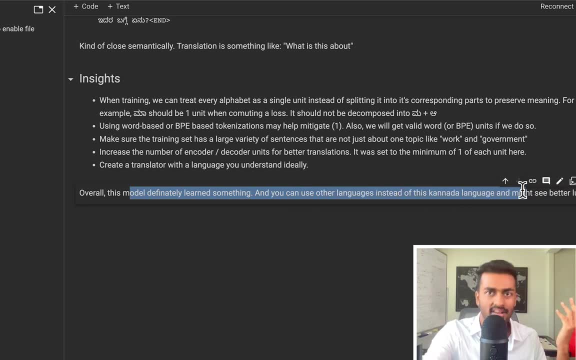 to pick up more complexities and intricacies in your languages. Overall, yeah, this model has definitely learned something and you can use it, for you know other languages in the set of Canada as well, So I still hope that this, all of this-